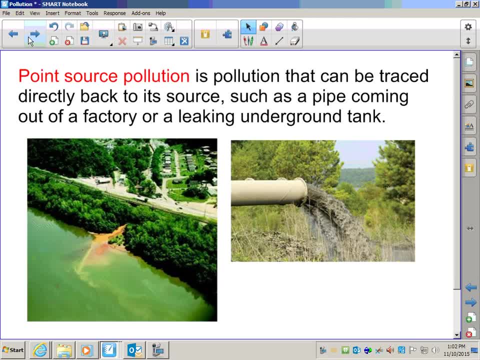 So you can trace the source of pollution: from a pipe coming out of the factory or a leaking underground tank. If you look at this picture here, it doesn't take much imagination to know that there's something wrong upstream from this little creek and that there's some sort of pollution that's running into. 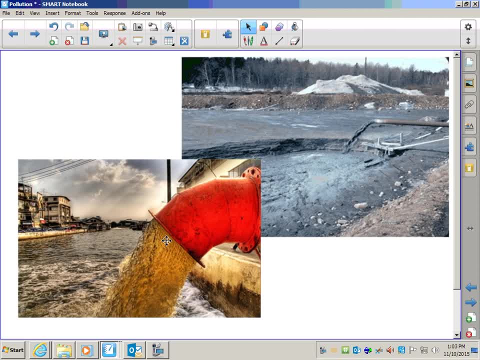 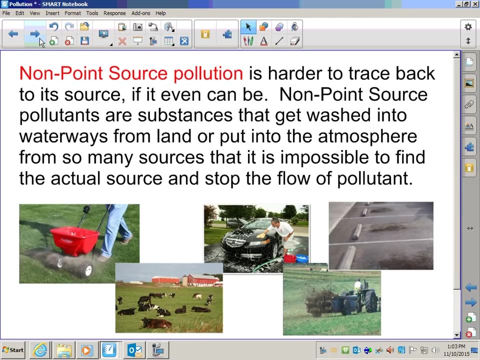 this river and this is the point of entry. Same with this pipe or either of these. Pretty easy to follow the pollution back to the pipe that's discharging the waste and the pollution itself. So point source pollution is easy to find. You can follow it right back to its source. Non point source: 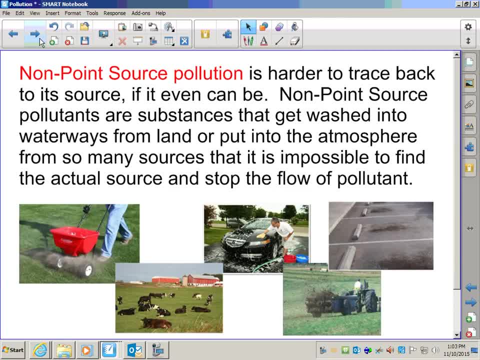 pollution, on the other hand, is a little bit more difficult. Non point source pollution is pollution that comes from pretty much anywhere. It can run into waterways when it rains. It can blow into the atmosphere from so many sources that it's it's really tough to know. Here are some examples: Fertilizer spreading or 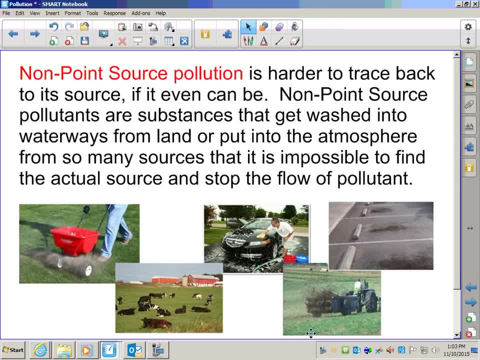 manure spreading can get washed into lakes or rivers when it rains and cause algae blooms. Same thing with soaps you use to wash your car in the in the driveway. That soap is a fertilizer and it can get into waterways when it rains. 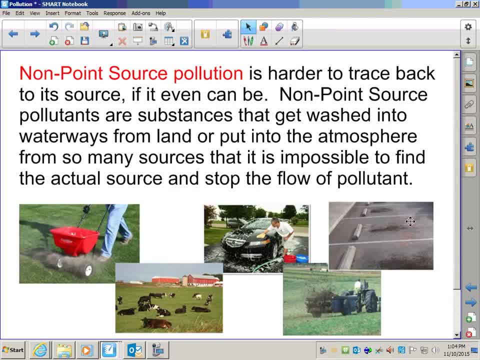 Who hasn't seen these blotches of oil in a parking lot? and when it rains they can run off into the storm sewers and ultimately into waterways, where they collect and pollute those waterways. The thing about non point source pollution is that it's so hard to find a direct cause that it's really tough to fix. 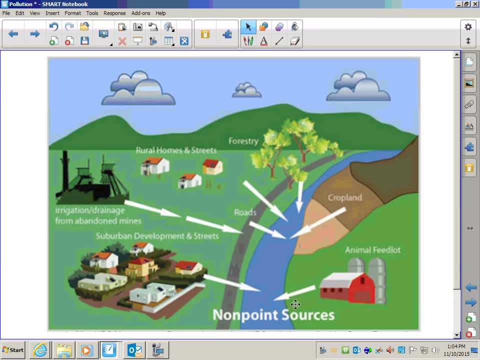 Here's a chart that just shows a few of the non point source pollutions: Cropland- either manure or fertilizers or chemicals sprayed on croplands can get into waterways. Animal feedlots can provide nutrient runoff from the manure. 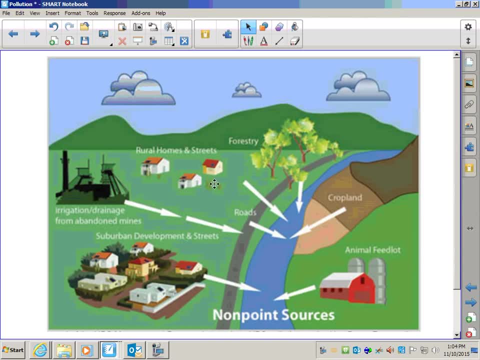 Homes and streets, and either suburbs or rural homes, can have things wash off or wash into waterways. Forestry and the disturbing of the soil allows sediments into waterways. Plowing fields for cropland does the same thing. Road salt and oils can get.